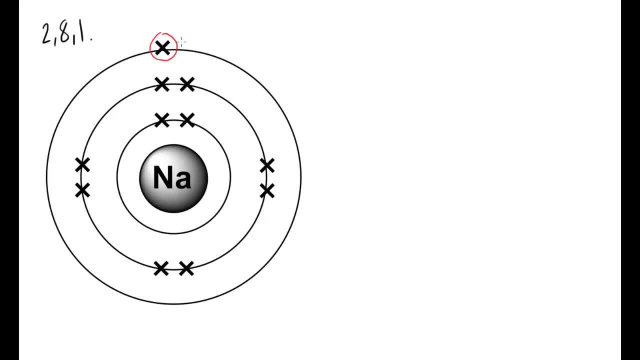 Each of these, each one of these crosses, is, of course, an electron, and in this case we have 11 electrons present, So 11 electrons within this atom. here Now, a few things about that, So a few things about the rest of this diagram, really, Leading on to a later point. really, These, each ring, is equal to an energy level. 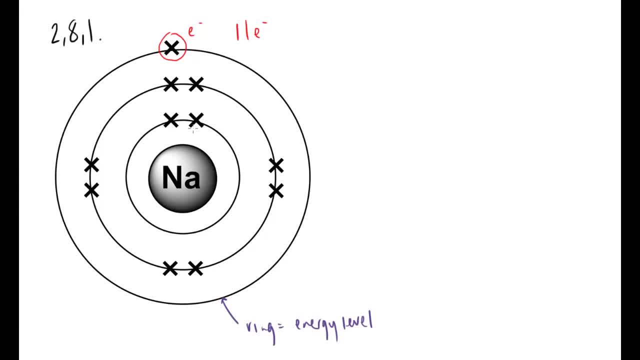 And in this case you can see that we have three energy levels, So three filled energy levels: First one here, second one here and third one up here. and that's the important thing really is the order in which these are. The first energy level is the current energy. 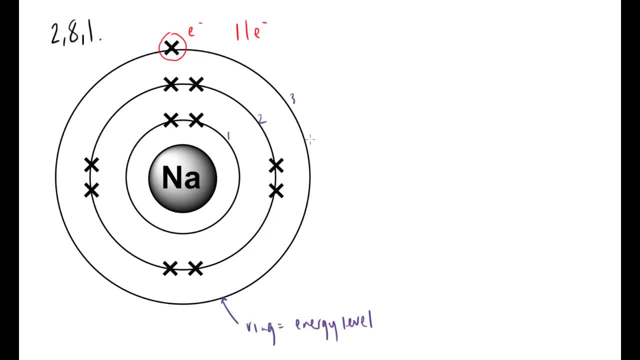 one closest to the nucleus, the second is the next one up, and the third one is the next one again. right? so what else is this diagram showing me? so i've got electrons, i've got electron shells, or energy levels as they can be called. um, i actually put this here. shells is another way. 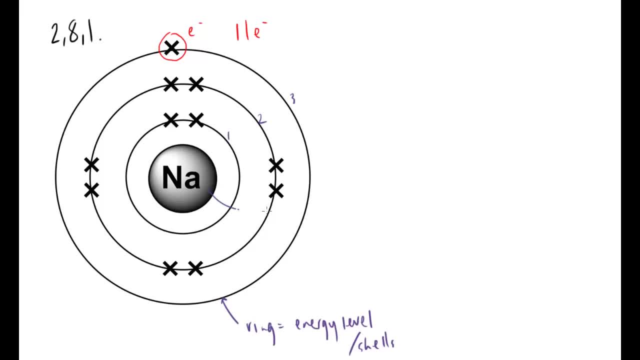 to word that, other things i've got. well, i've got this thing in the middle here i've got a, a nucleus. now a nucleus is fairly important. it's the, it's the center of the atom. it's this incredibly, incredibly dense in relativistic terms to the rest of the atom, where almost all the mass of 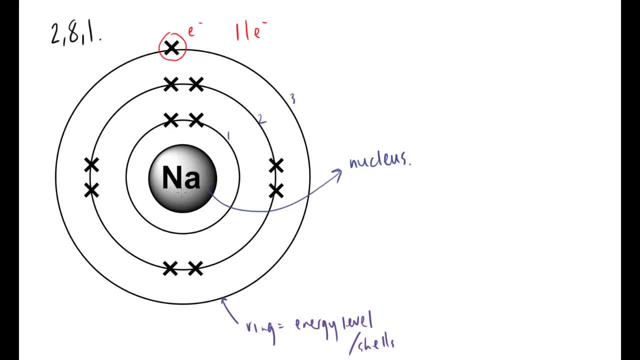 the atom lies in this very central point and then in between the electrons. in here we just have essentially empty space, which is a strange idea. but there you go. nucleus. this is made of protons and neutrons, and what we find here is that protons and neutrons- well, each one of these- 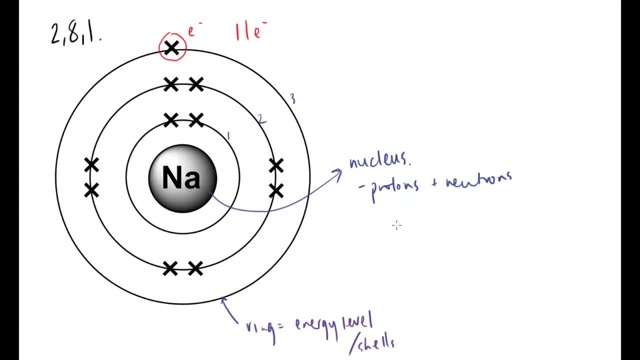 it's kind of- i'm going to say quite a lot in this short space of time because i feel it's gcse and therefore there's not really any need to sort of dwell on it. a huge amount protons and neutrons. they give us the- uh, the mass number. 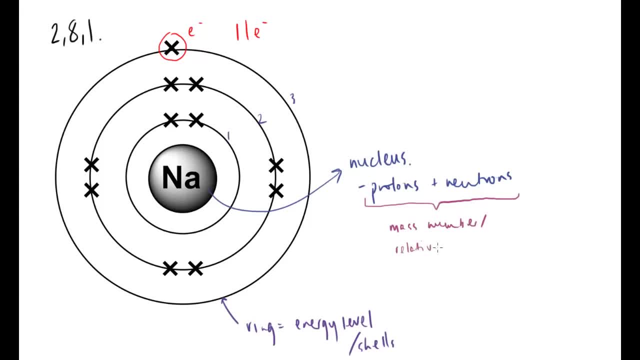 or better terms, uh, the relative atomic mass of an element, and you'll see that in a periodic table. so in the case of sodium, um, i'll try and remember what it is now. i think it's na. uh, i think it's 23.1. i think it's 23.1. 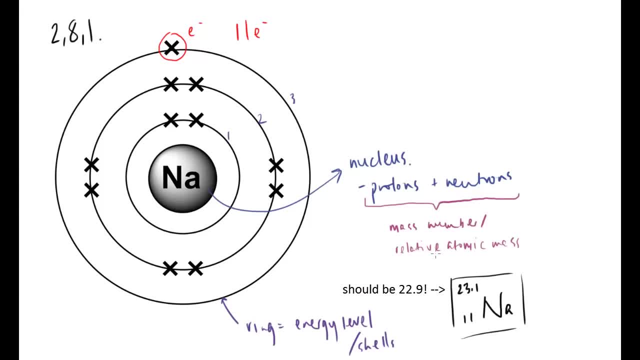 one and eleven. that's what its little square on a periodic table would look like. um, and in this case, the relative atomic mass. is this guy here? okay, this top, the bigger of the two numbers which leaves, is a bottom number. now, this bottom number is the atomic number, and in atoms, 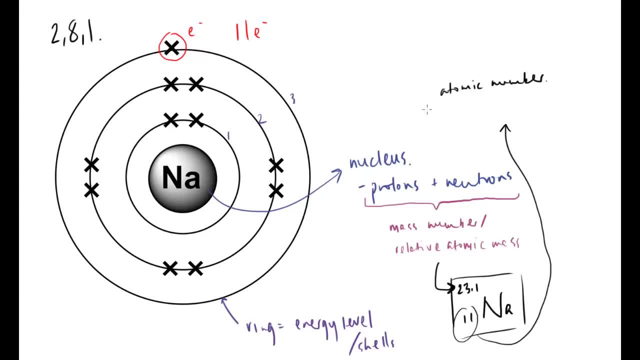 atoms, not ions. atoms, the atomic number is equal to proton number and that is equal to the electron number. and that's why i'm saying atoms. here we're dealing with ions, we're changing the numbers. it doesn't work: proton numbers and electron numbers is the atomic nutter, atomic nutter, atomic number. 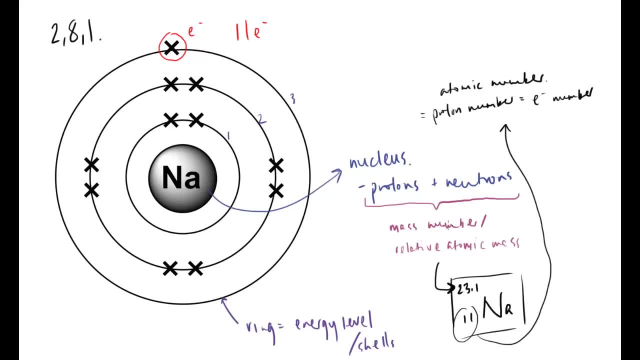 so a couple of bits, protons and neutrons. well, they equate this mass number, the reason being that each one of these has a relative mass of one. so relative masses of one. electron, we can say, has a relative mass of approximately zero. it's about one over 1187 or something, but it's. 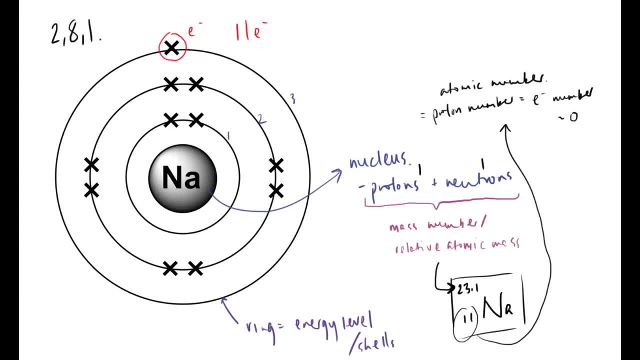 about one over 1187. so we have zero. so again, relative terms, it's zero charge-wise. why does the? why do the number of protons equal the number of electrons? well, charge-wise, overall, atoms have zero charge. so atoms are neutral, a better way to say that. 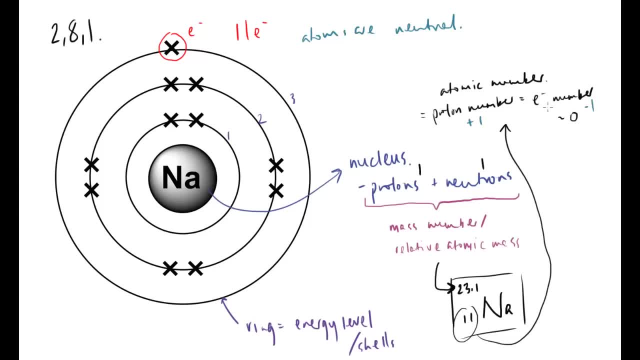 and that's because protons have a charge of plus one, electrons have a charge of minus one and therefore, when they're equal, we have a zero charge, the other thing being neutrons have a charge, therefore they have no effect. so that's quite a quick, quite a big uh, quite a quick, uh, sort of. 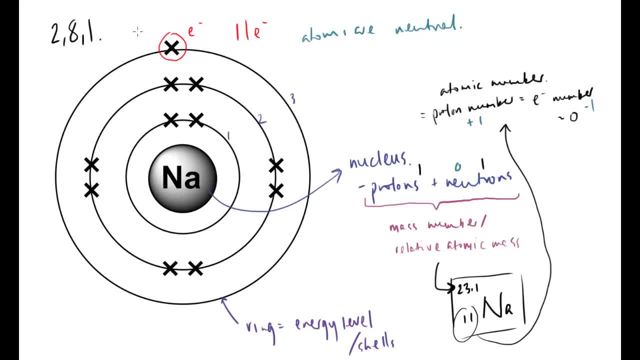 recap, i guess, in some ways of sort of this idea of the atom. um, particularly then these, these electron configurations- and that's what i now want to spend a bit more time on- is these electron configurations, and and how we can develop that in a level, and why? this is a simplistic model. it's 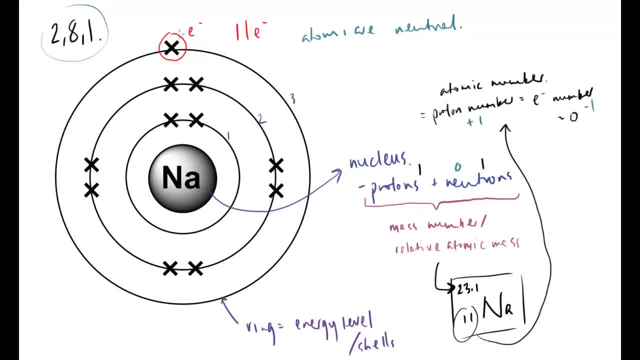 one that works the ball model. it certainly works in many ways and and it isn't strictly speaking wrong, but to the level you do it at gcse. there are a couple of um- not lies or fibs as such- but there are a couple of simple simplifications, and that's often why, when you're at gcse, you have to. 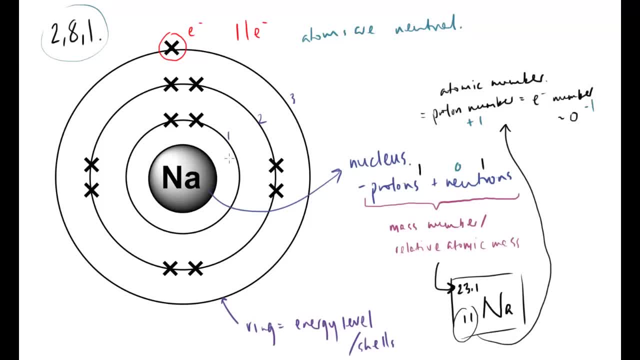 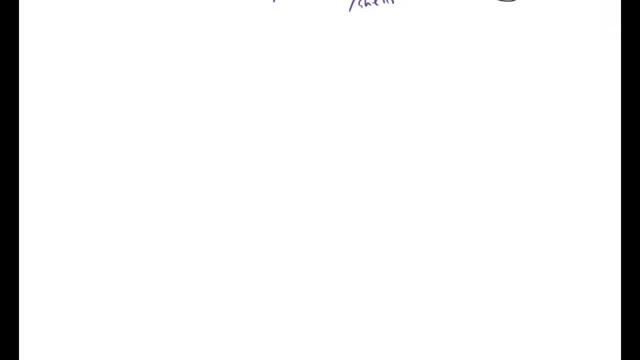 learn up to calcium. you don't go into the transition metals because at that point things get a bit weird, which hopefully by the end of this video you'll have an understanding of and you'll know why they get weird and actually why there's a lot for people. aqa chose to stop it at calcium. 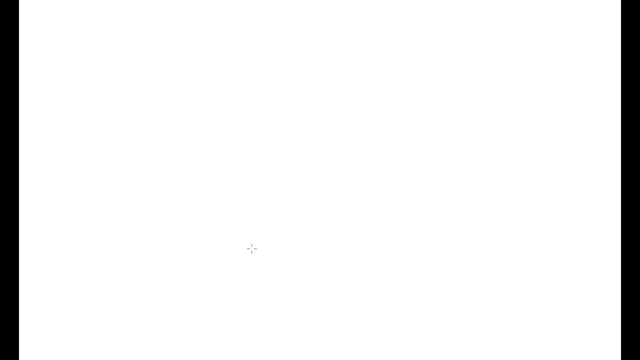 rather than move into um. i forgot the next scandium, i think is the next one, uh, and then titanium, um, so they stopped calcium for a reason. so electron configurations: now, as we've already seen here, and this is true- that electrons exist in energy shells. so we have energy shells, or we call them energy levels, or actually we'll go energy levels slash. 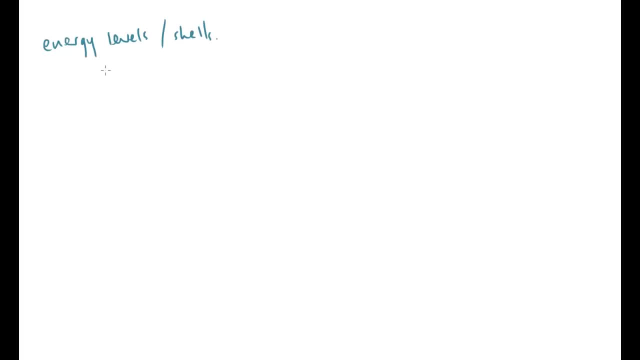 shells best of both worlds and they can be anything from. they're often given, that's given the symbol n. uh, you're not really really to know that um, starting on the inside, we can go one, two, three, four. that's probably about the extent that you're going to get to in um in the as not. 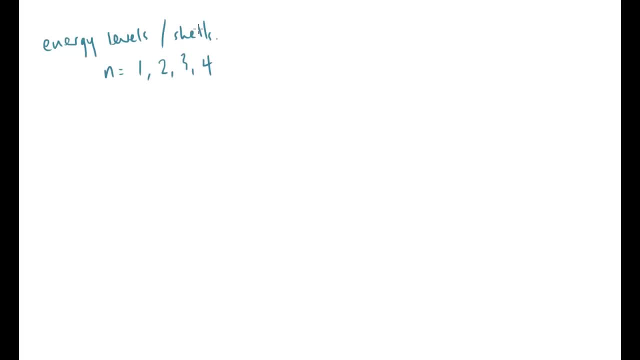 going to get any further than that. so we've got four energy levels, or a a bigger number, but four is just what we really need to look at. i warn you at this next point you're probably not going to have a clue what's happening. but the best way i'll ever teach this i i find that people just 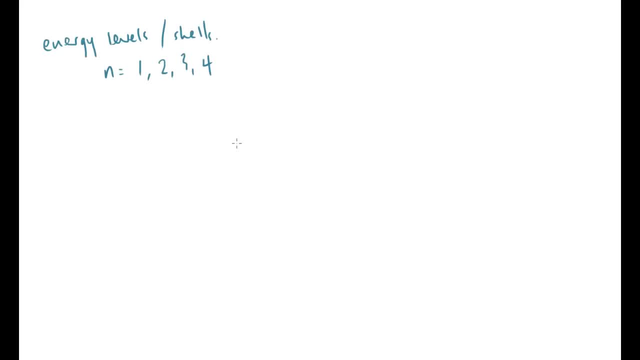 kind of get really confused, but hopefully it's sort of the penny drops towards the end. there's a lot of weird information about what's going to happen in the future, so i'm going to give you a little bit of information, and it's difficult to know what order to do things, but hopefully this 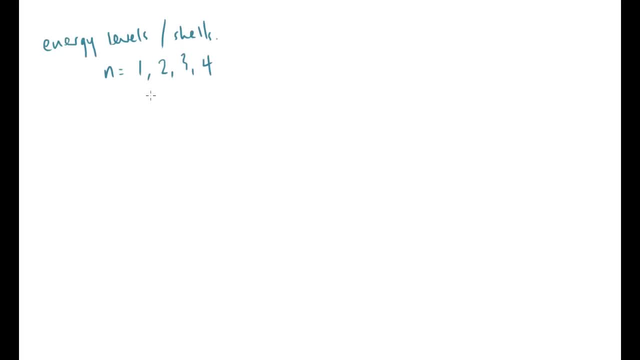 will make sense. so electrons are found in energy levels. now each one of those energy levels is split into what's called sub shells and they are given the letters s, p, d and f. that's a fairly strange idea, but even more strange than that, each one of these is split into orbitals. 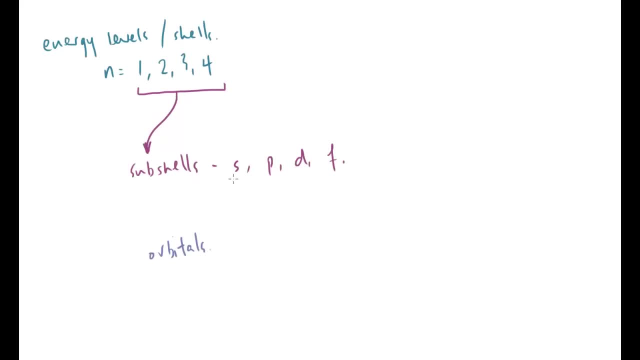 and these orbitals work as follows: the s is one orbital, the p has three orbitals, the d has five orbitals and the f has seven orbitals, of which you don't really need to worry about. f is, um, an annoying one really. we can just kind of exclude that for the sake of the, as sp and d are what you. 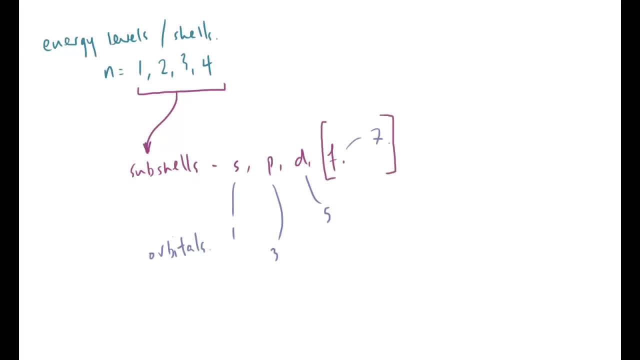 guys are going to be looking at. and then slightly easier one. here each orbital is called two electrons. note that i mean each orbital, not each sub shell. so actually what it means is that um s equals two electrons because it's got one orbital. p equals six electrons. 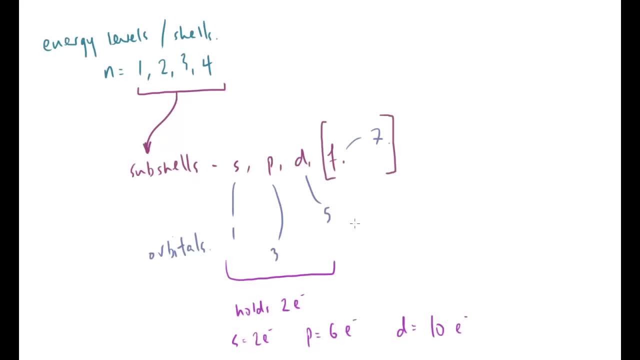 because it's got three orbitals and d equals 10 electrons because it has five orbitals. now, at this point you are not going to have a clue. i would guess what's happening in it. the whole thing just seems very strange and you have no idea where these sub shells have come from all. 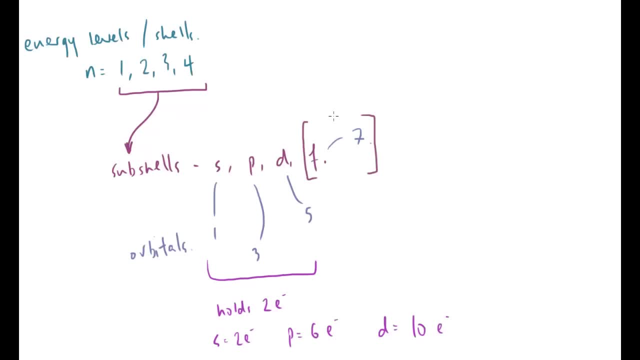 orbitals and all the rest. now there's this. this whole thing can get quite difficult when you start thinking about electrons and all the rest, and so I don't want to go into a huge amount of detail as such. more that the orbitals really are when we think of electrons, the idea of this Bohr model implies that 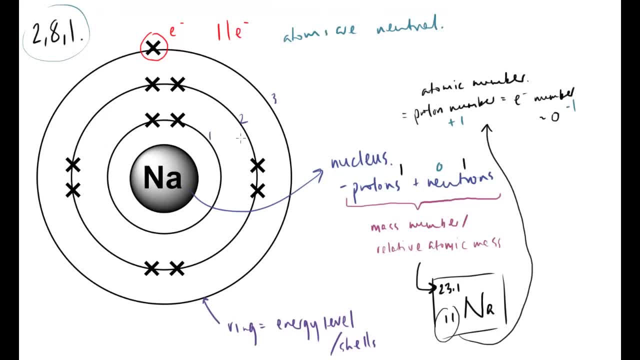 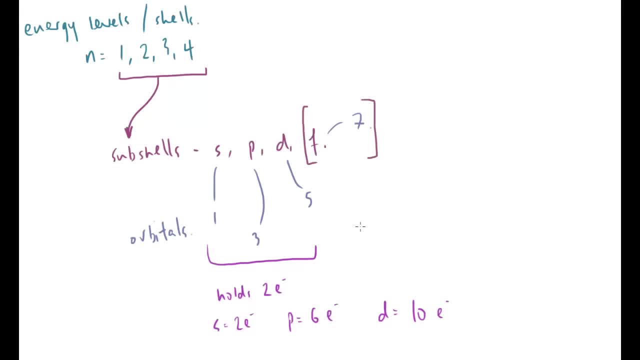 electrons are very static, they're just so. that they're orbiting is another idea. electrons orbit the nucleus, which isn't really true. the electrons can exist in, really, as far as I'm aware, sort of anywhere they really want to, and what these orbitals do is the orbitals are really the the place where you're most. 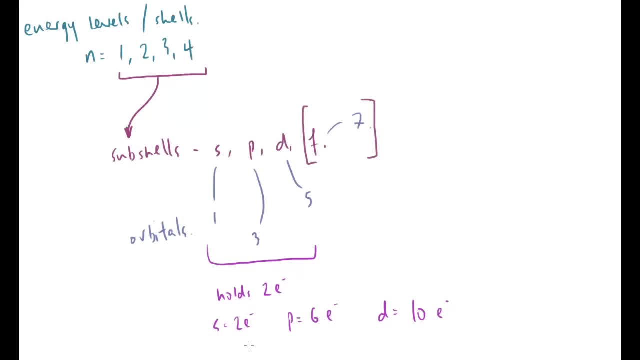 probable. I think there's something like a 95% chance that the electron will exist within this area of orbital. so it's, it's an area of the atom really the orbital is, and that it's the area where the electron is most likely to appear. now you 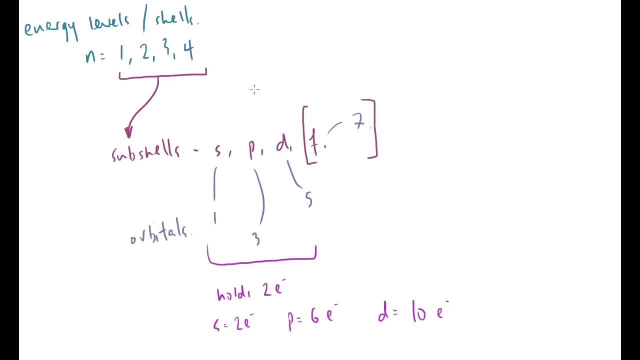 don't need to know that an exam in terms of an exam, we have to be able to do is use this to write an electron configuration for an atom or for an ion, but don't have to worry about the reasoning behind it. but that's really kind of it. the orbit, the orbitals are where the electrons are. 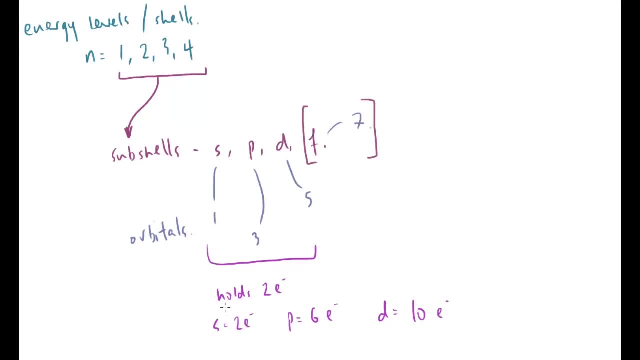 are most likely to be found now. if you want to look this up, chem guide's got quite a good explanation on on orbitals and all the rest. i don't want to go into details for it because i'm looking to sort of cover this for the masses, as opposed to those people who really want to go. 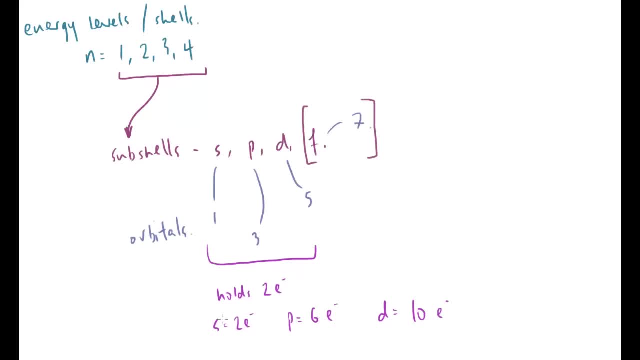 into sort of quantum, quantum land and do all various bits. i don't want to be there. to be quite honest, i'm quite happy here and so i'm going to leave this at this and i'm going to add one more thing to this and then i'm going to actually look at sort of what we're doing. in fact, i'll put 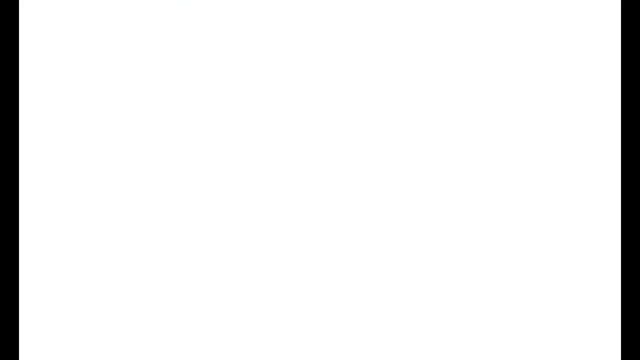 that next bit down here, and then i'll give you some examples of stuff. final thing i want to add on or point to this is is the order of which things work. so the first energy level has an s subshell, and that's it. second energy level has an s subshell, and it has a p. 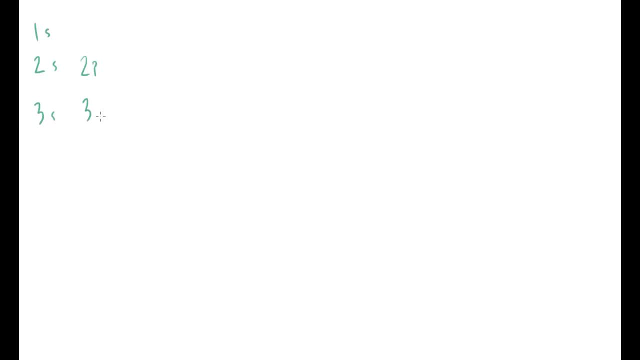 the third one- lets see where this is going to go now- has an s, it has a p and it has a d. the fourth one has an s, has a p, has a d and it has an f. although we're going to for the sake of this, we're. 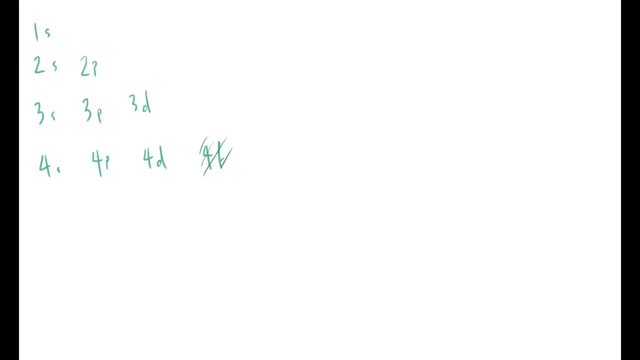 going to kind of ignore the fact that the energy level f exists. It's just needless confusion for now. So the reason I've drawn this diagram this particular way is because it's very important, because it tells us how these things fill, And I will give some examples. so this should hopefully make sense. But as I said at the 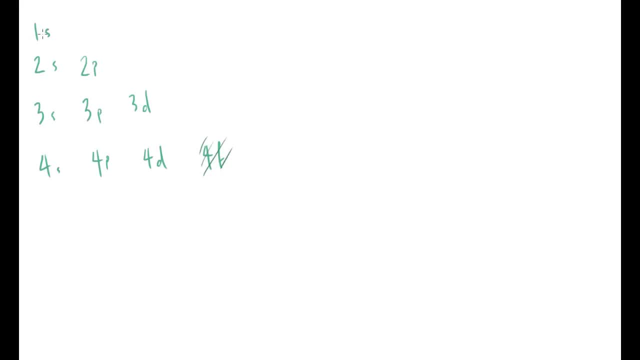 minute. it's perhaps just very confusing, but bear with me. The electrons fill these things down. So I'm starting here. we go down, across across there, across there, across there and down. okay, And 4p is about this far you're actually going to get, I think, the furthest. 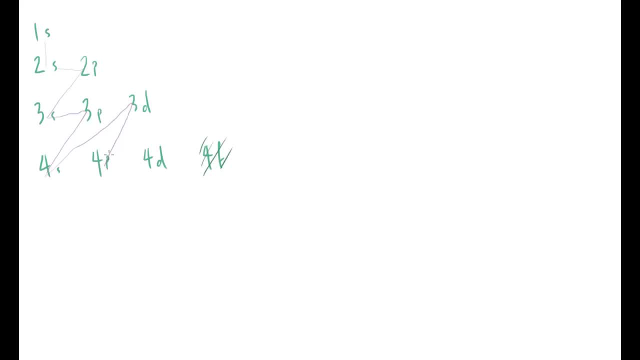 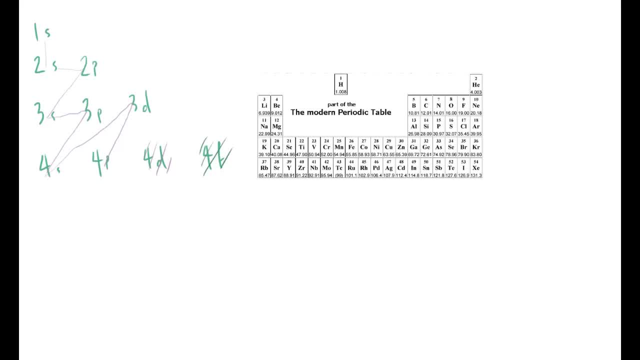 much because it may seem like the loved song. Don't you guys have aée or something? Well, when they 4P and if you look at a periodic table, this is because actually, what we find is that we separate the periodic table into particular areas. So this here, this is the D block. 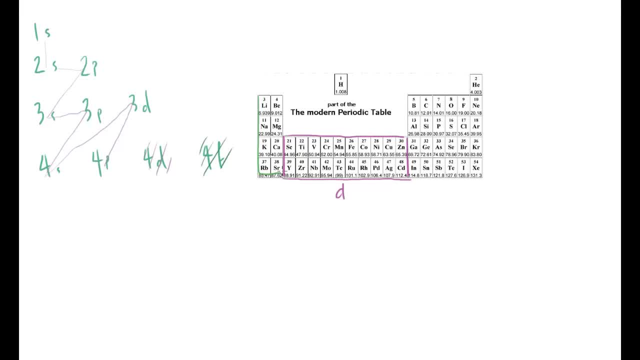 this up here. this is the S block and finally this one over here, P block. so S, P and D, And actually, if you start thinking about, well, what's going to happen when I'm actually going on these electrons, well, we start up here. this is going to be our 1S. it's going to 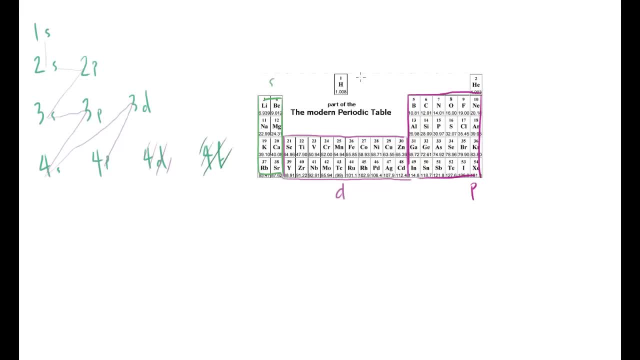 be our 1S, 2S. sorry, this is going to be one of the 1S's and this is going to be the second 1S. We're then into this section. here we're adding the 2S and then we're into the 2P, 3S, 3P. 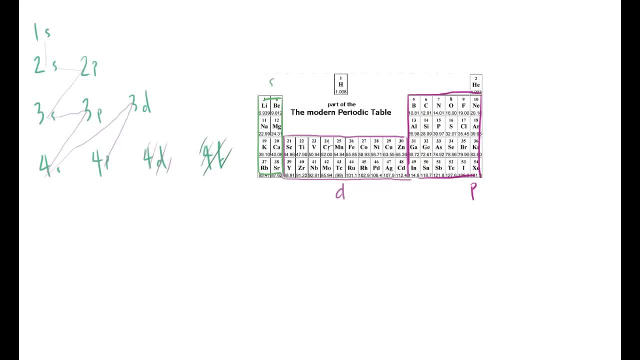 well, now we're into the 4S, but then it drops into a 3D, which is a new one, followed by the 4P. So we think about it in this section in this way. so we go 3S, 3P, 4S, 3D, 4P, and then 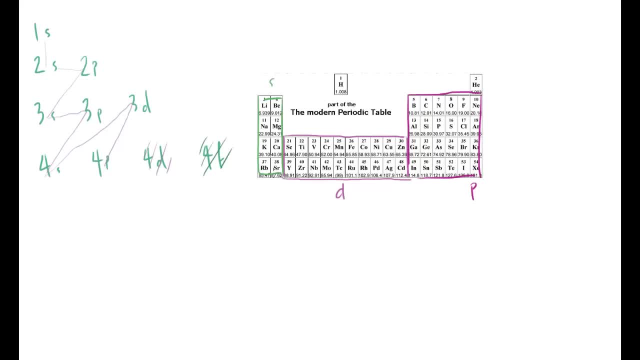 it would then go 5S, 4D, 3P, 5P, and actually you end up with the F I think comes in about here. it might be one lower. I forget where that exactly squeezes in, But you are expected to know this is the S block, this is the D block and this is the. 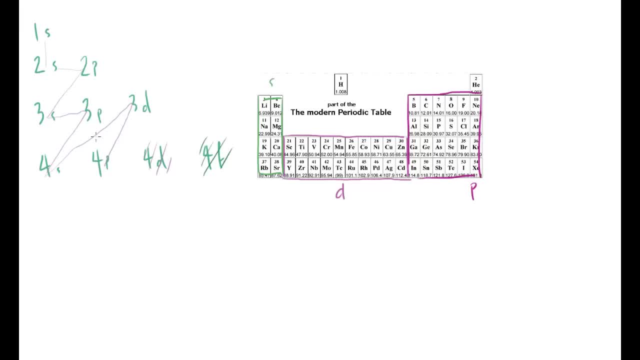 P block and that occasionally comes up. Now I'm going to do a couple of examples, because by this point I would guess some people are probably quite confused. this is actually how you would write out electron configurations for atoms or ions. So say, we've been asked what the electron configuration is for sodium. 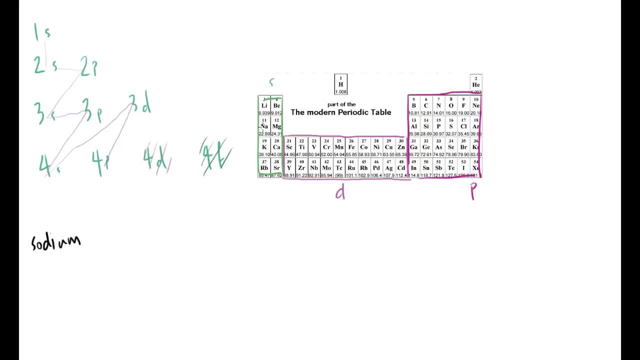 Well, We've got sodium in our periodic table and we say, oh, here's sodium, right here. we can see it has 11 is its atomic number, and therefore we have 11 protons. therefore it has 11 electrons. So the 11 electrons. what do we do? 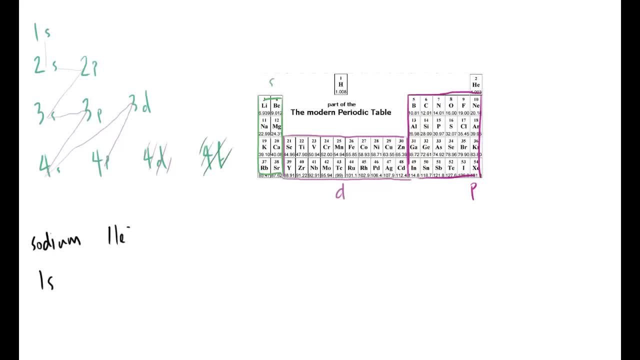 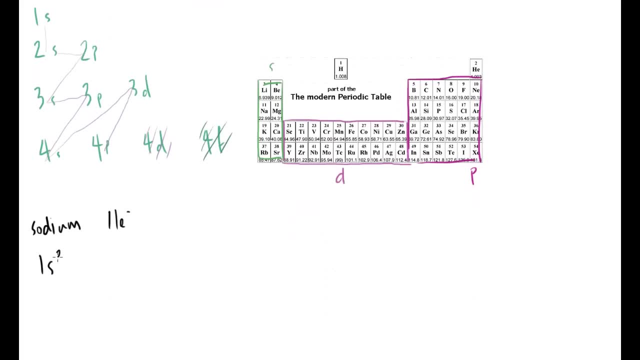 Well we go, we start at our 1S. Now we know that our 1S can hold 2 electrons because it has 1 orbital and in this case, it's going to hold all 2. and that's what this little number here tells you. it tells you: 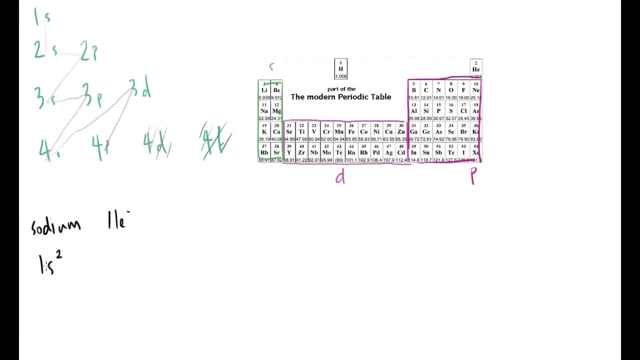 how many electrons are in this particular atom Subshell. So it's going to hold both of the 1S. it's going to have both of those electrons there. It's also going to have both of the 2S ones as well. 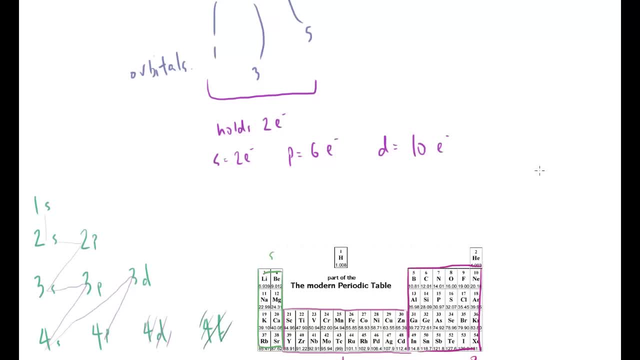 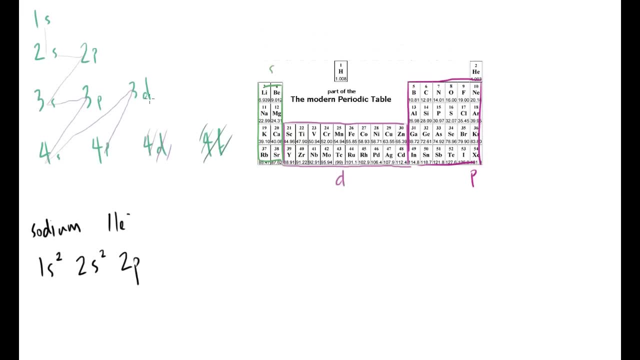 Remember the S, just because it's 2S doesn't change. S can only ever hold 2 maximum. We move into our 2P this one here. scroll this up slightly- move into our 2P. so we've. 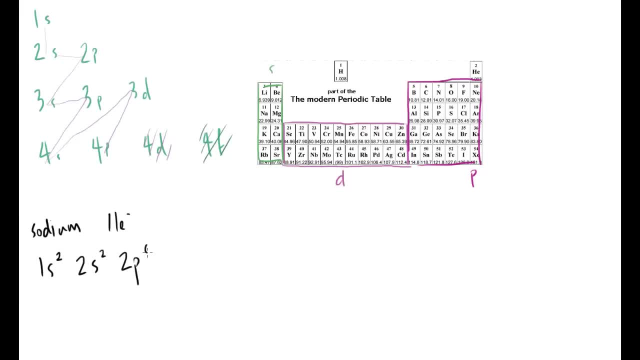 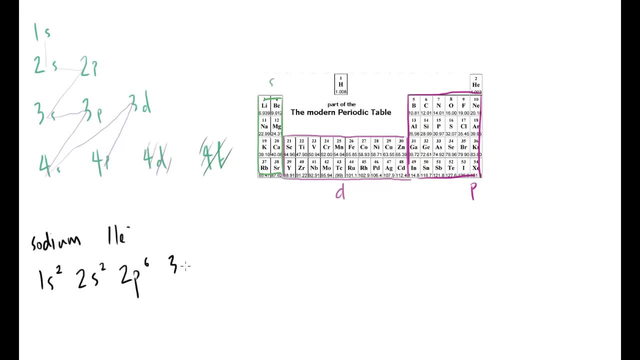 gone 1S, we've done 2S, we're now at 2P. well, it's going to hold all 6 2P electrons, remembering that P can hold 6.. And then, finally, we're now into 3S, where we're going to add our 1.. 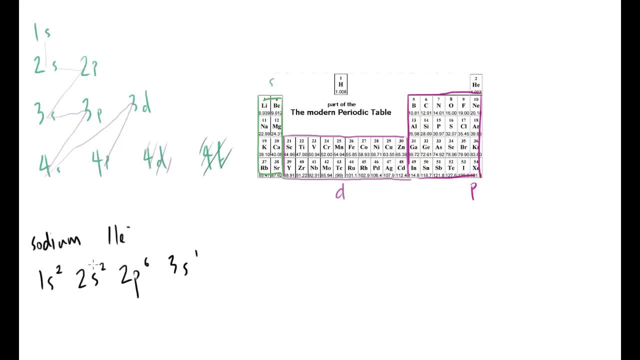 Now the numbers here: 2,, 4,, 10,, 11, this is our. these little numbers are telling us the electrons in subshell. Okay, so they're telling us the electrons that are in the particular subshell. So 2 in this subshell, 2 in this subshell, 6 in this subshell, 1 in this subshell giving. 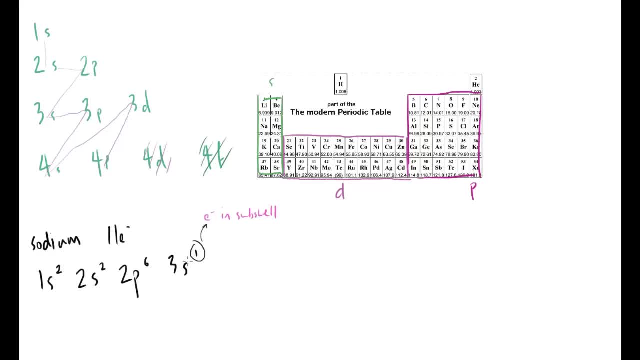 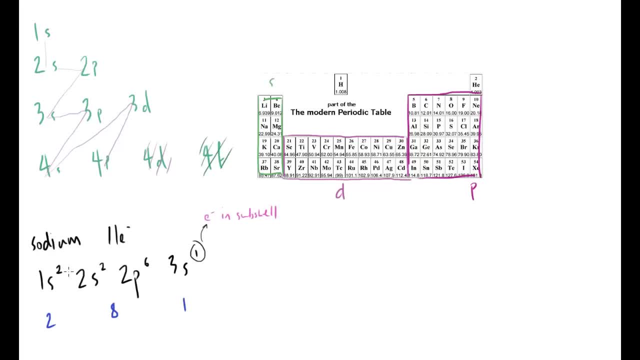 say: well, actually this is where the 2, 8, 1 came from, because this here is our second energy level. this is our first energy level, so you can see 2,, 8, 1.. So that wasn't a complete lie. it just didn't take into account the fact that we have the 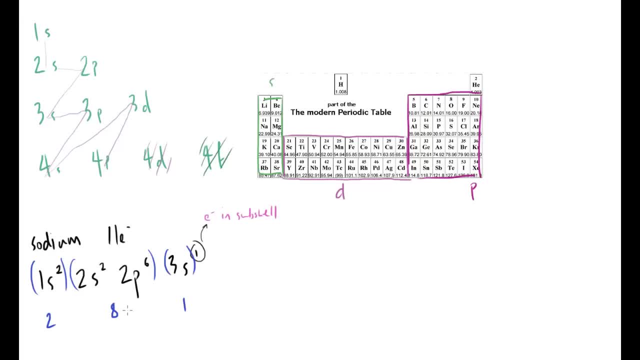 subshells within the energy levels. it just takes into account that the electrons exist within an energy level- Another way to look at this- and you are expected to know this in an exam, sadly, Okay. So what we're going to do is actually: the orbitals are drawn out as little boxes. 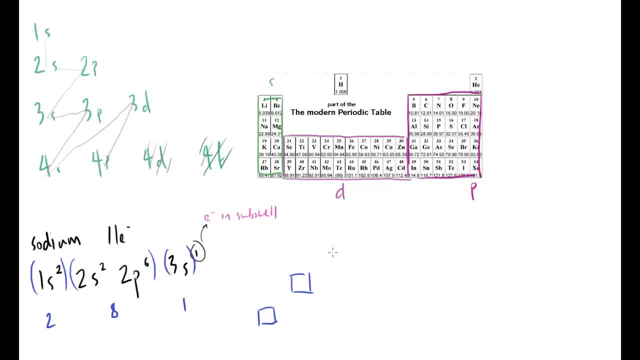 So we have a 1S orbital here, and I will label this up in a second so it makes more sense. So what this is doing is this is showing us the 1S orbital. this is the 2S, this is the. 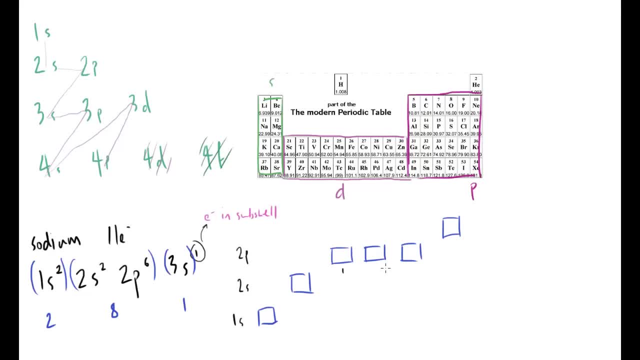 2P or subshell, I should say, this being the first P, second P, third P and this here being the 3S across there. What happens is we fill as is. I didn't make this up. by the way, it's called the bus seating. 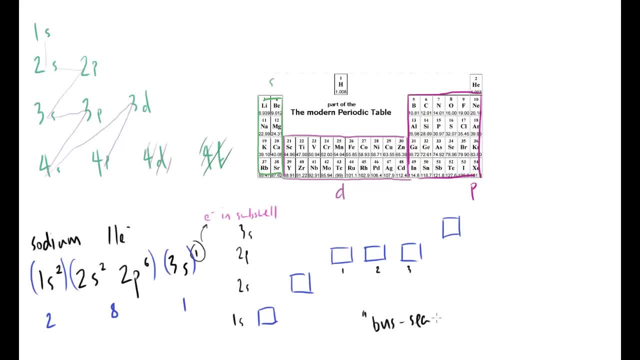 rule And if you can remember the bus seating rule, you will remember how to draw these and occasionally you have to fill in these diagrams to show the electrons in the orbitals- the bus seating rule, And it works as follows: if you imagine getting on a bus or a train and you've got a load, 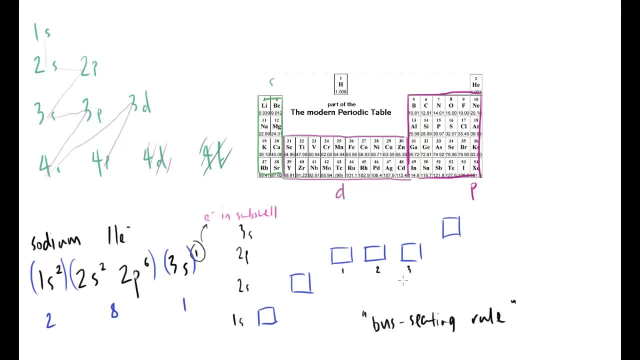 of double seats, Each one of those double seats representing an orbital. You don't. if someone's sat in a double seat, you sit in the next empty double seat, don't you? You don't then sit next to someone. So the bus seating rule is that everyone fills the empty double seats and people only double. 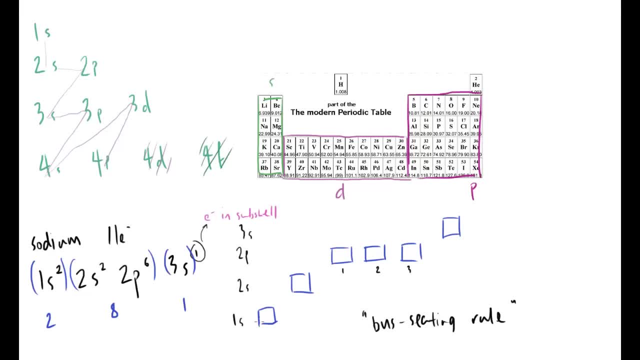 up. once the seats have one person in, Once all the empty seats are partially filled, that's when people start to double up seats. They do not double up straight away, and the same is true of this. We fill in order, So we do our 1S and then our 1S. 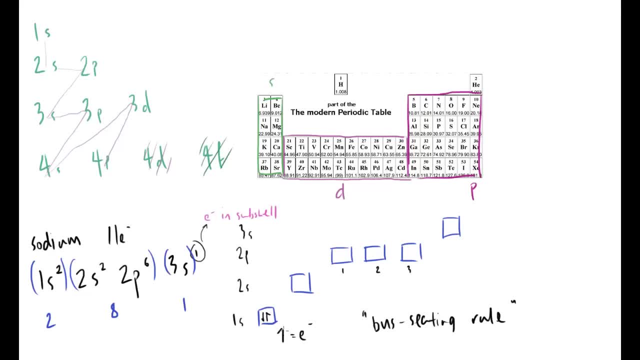 Know that each one of these equals an electron. The arrow is just denoting the different spin. So that, and then that is what I've drawn in there. You must in an exam draw them other ways round. So, single headed arrow, one pointing down, one pointing up, doesn't really matter about. 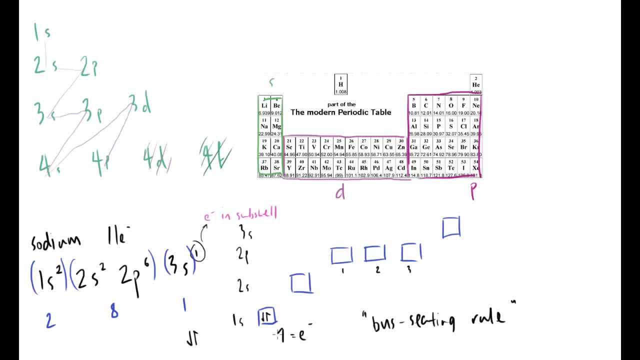 the order. just one must be pointing down, one must be pointing up, and that's to do with spin. Just know that that's what you do, Don't worry about understanding that. So 2S. well, now we've got two in our 2S so we can fill that up. 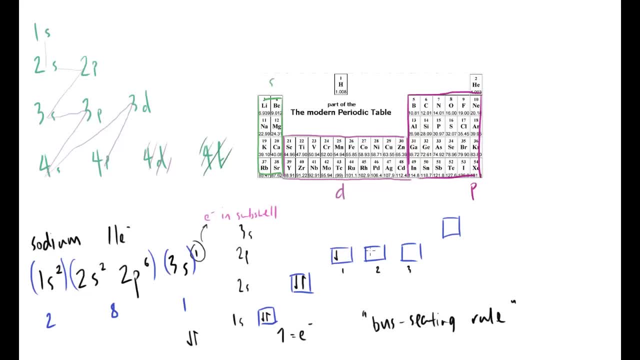 Our 2P. well, we know, we've got one. See what I mean by the bus seating rule. It would fill in this order: one and then one and then one. Oh, now the next person's got to join up. we've got to join up, we've got to join up, and. 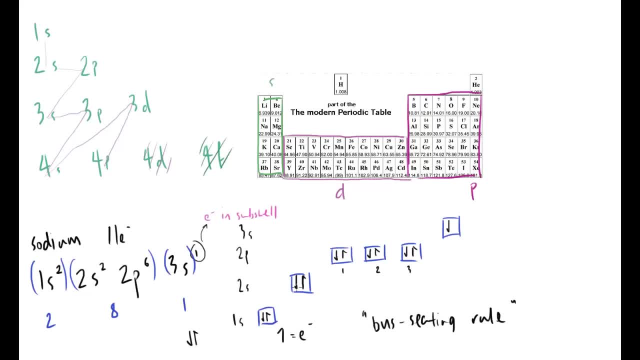 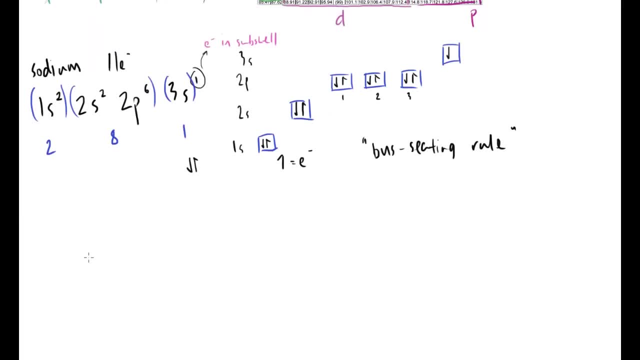 then, finally, we have our 3S1.. So there we have 1S2, 2S2, 2P6, 3S1.. Do another couple of examples. We'll do oxygen, and I've chosen oxygen for a reason. 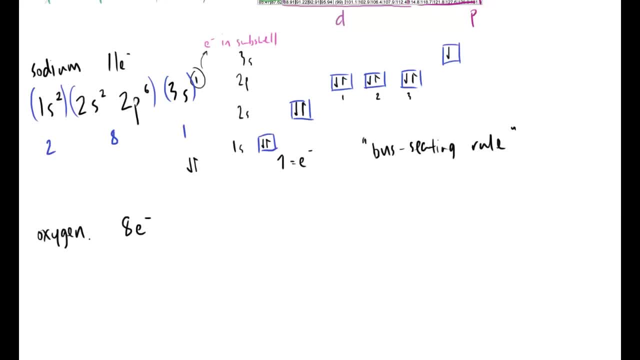 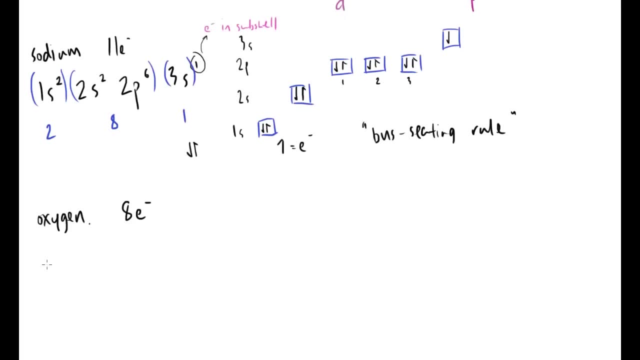 Oxygen. We've got 8 electrons. We can see that up here- Oxygen 8.. So 8 protons, 8 electrons, Which means we go through the same order as before We start on our 1S. Well, we can have all two, that's fine. 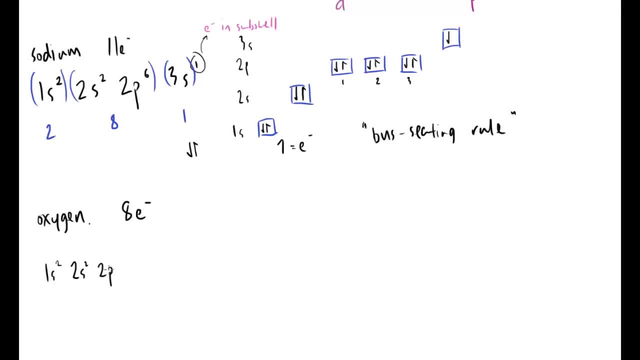 We go to our 2S. Yes, we can have all two. We go to our 2P. This time we're not going to fill our 2P because we've already got 4 electrons out of the 8. We've got the other 4 to put in. 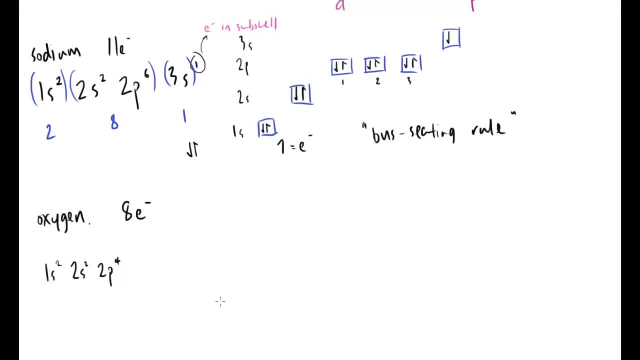 They go into that P there, so we have 2P4.. And if I was to draw my lovely little diagram, as before, The reason these are drawn in different levels, by the way, is just denoting energy. This is a scale of energy really increasing energy. 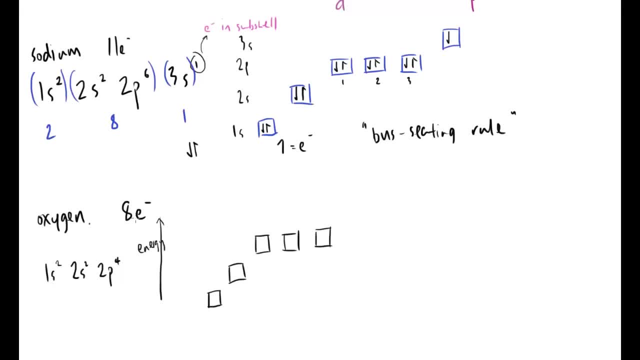 So this is at a lower energy than this And that will make more sense as you go through, particularly when it comes to periodicity. But write this very second, just worry about how to sort of fill these and write these electron configurations. So we've got pairing here. 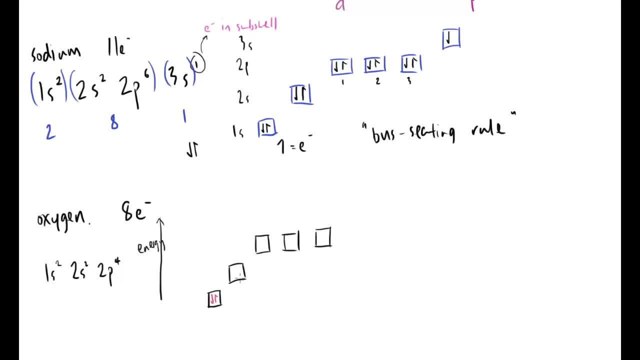 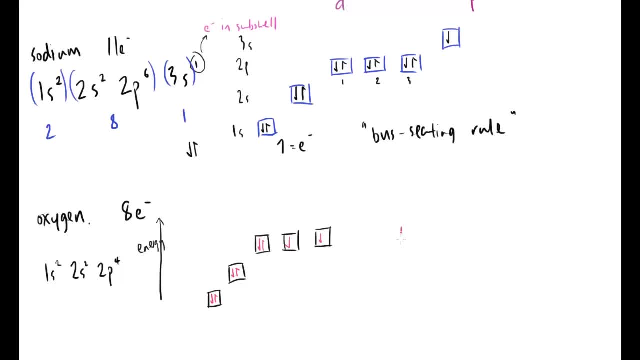 And they quite like this in exams, because what you might see some people doing, some people might write it out as this, which, by the way, is wrong. They might go: oh 1,, 2,, 3,, 4, and leave this one blank. 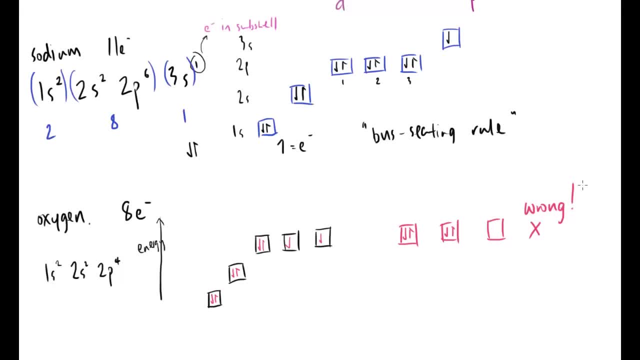 That is wrong on so many levels. This is correct, this bus seating rule: we have single fills and then we double up, and then we move to our next one. we single fill, double up, then we move to our next one, blah, blah, blah, blah, and we keep going. okay, um, i'll go for another one, just to. 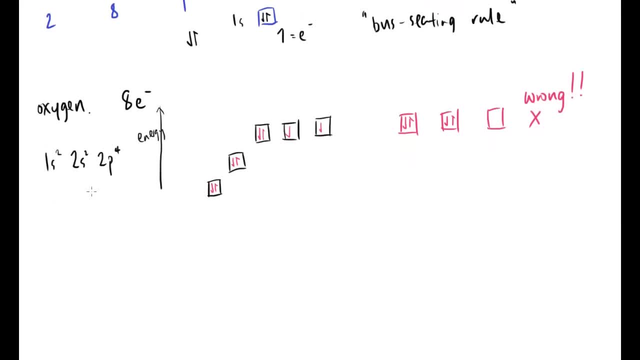 take a bit further and we'll do titanium, because we've done some fairly tame ones so far. we'll go into that d block now. so titanium: if you look on a periodic table here and hopefully titanium is on here, yes, it is 22 then we're looking at. so 22, let's have a go at titanium. 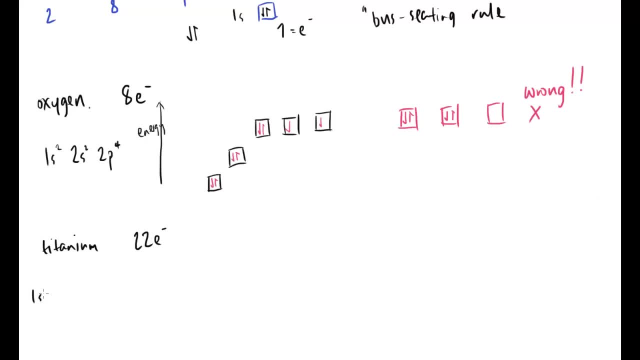 22 electrons. here we go, so: 1s2, 2s2, it's going to be 2p6, it's going to be 3s2, it's going to be 3p6. now, at this point, we have filled across, we've gone: 1 electron, 2 electron. 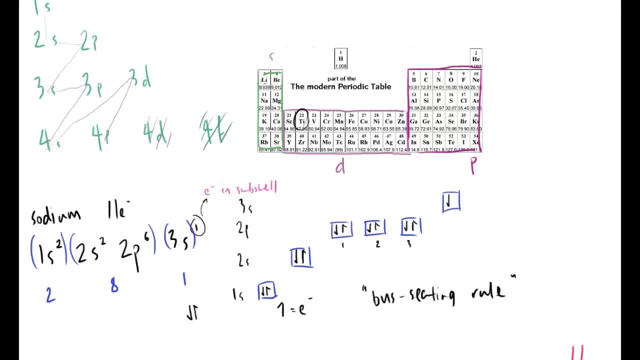 1s2, 2s2, so 1s1, 1s2, 2s1, 2s2, 2p6 takes us to there: 3s2, 3s2, 3p6, and we're now here. at this point this is our 4s part. so we're now into the land of 4s and we 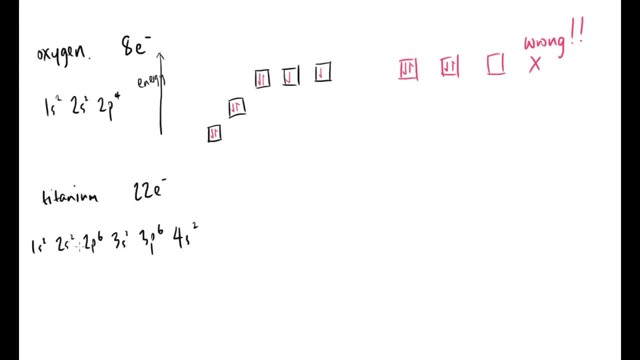 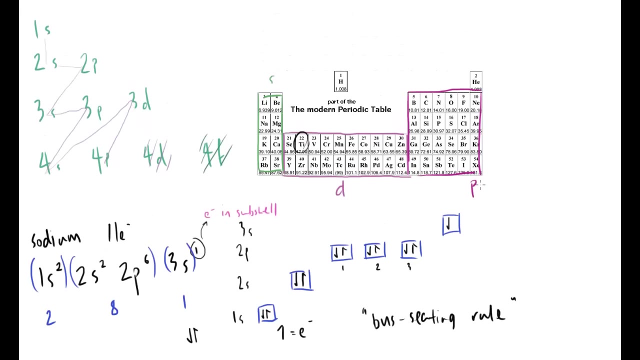 can fill both of those 4s electrons and we've got 2, 4, 10, 12, 18, 20, two more to put in and that's 3d, 2, no different. before sticking to our um, this thing here, 3p, 4s and then 3d, key thing is the. 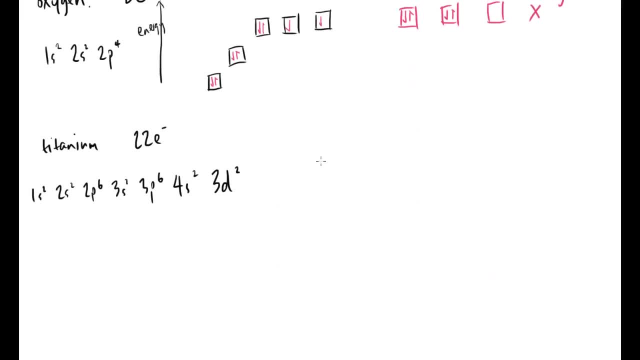 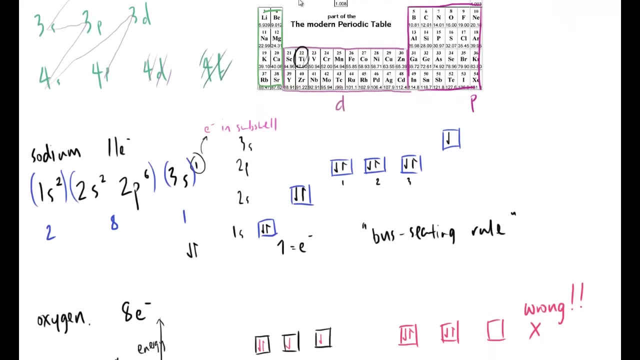 4s fills before the 3d, absolutely imperative. there is a shorthand way of writing these and which you may see at times, and the shorthand way of writing this electron configuration is as follows: the reason you've got ar in brackets is because, rather than writing the whole thing out, 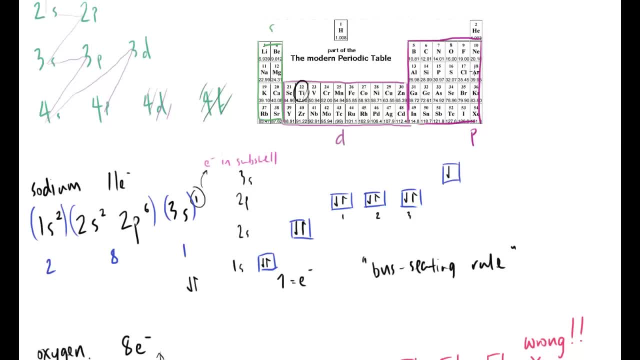 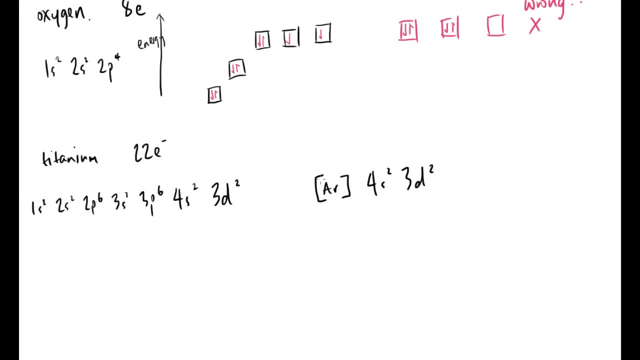 what you do is you assume that you've got the electron configuration up to and including argon, which accounts this whole section here, and then all you have to add on is the one, two, three, four. so we've got argon. then we just add on the one, two, three, four there. so it just makes it a bit. 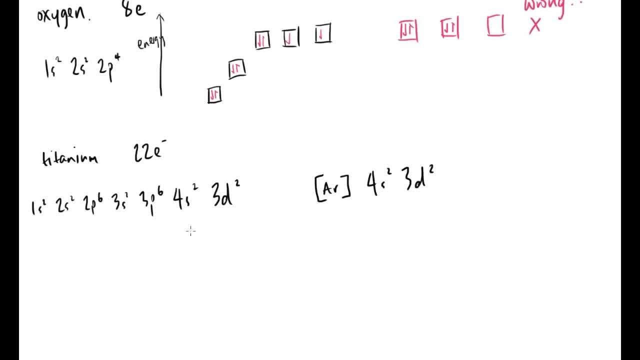 easier. i would stick, if you can, to the the full long one, because it's not going to take you a huge amount of time to write. this is okay and often it's accepted unless they use the term full electron configuration. but to be honest, i would. i wouldn't risk it. i would go with this, but you may. 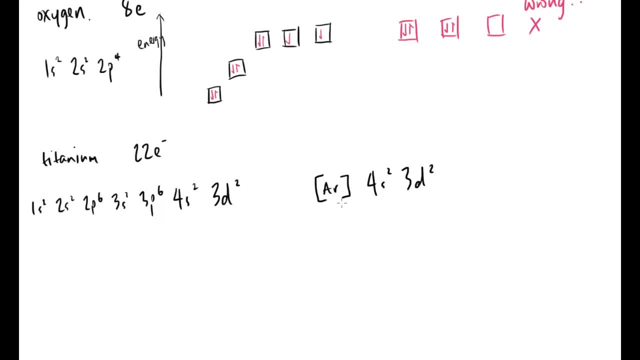 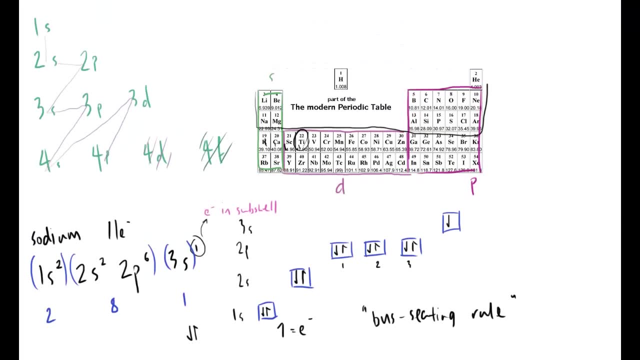 at times, see this given, and that's just that's why i've shown you that there. titanium, um. the other thing is to look at, obviously, if we had ions, um, so we've got the electron configuration and we've got two electrons. so let's have a look at magnesium, so magnesium's 12. 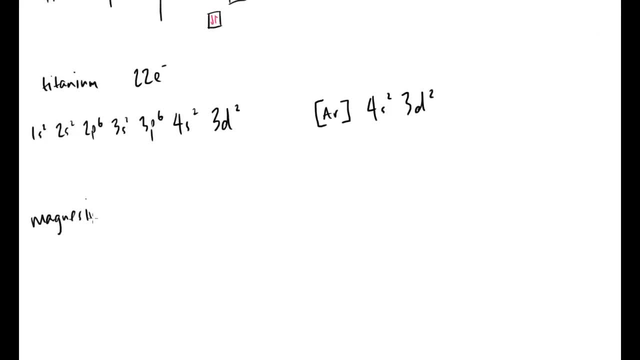 magnesium, 12 electrons, and so we fill 1s2, 2s2, 2p6, 3s2, 2, 4, 10, 12. that's fine. now if we were to look at the mg2 plus ion, that, on the other hand, now has lost two electrons because it's lost two. 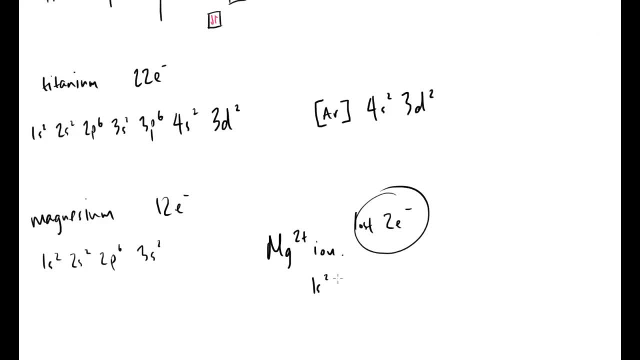 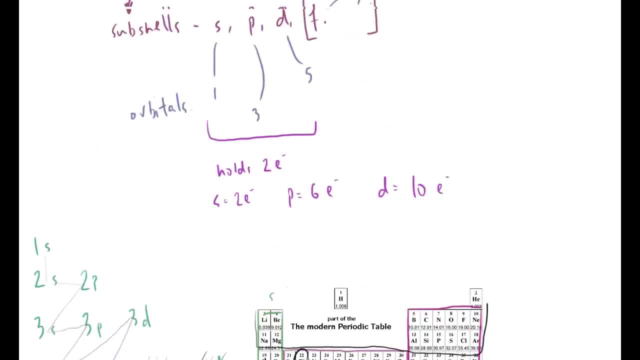 it's going to lose these two. so the magnesium ion is now 1s2, 2s2, 2p6 and that's it done. it does not have those 3s2, and if we were to fact to think about that in terms of our original diagram here, 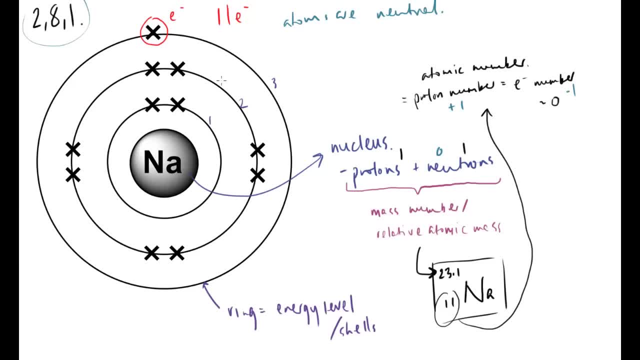 what that equates to is losing both of its outer shell electrons because, remember, we number or name whatever from the first shell outwards and so when we lose them, we lose from the outer shell inwards, these being the last two that we lose. and that comes up again in um in ionization. 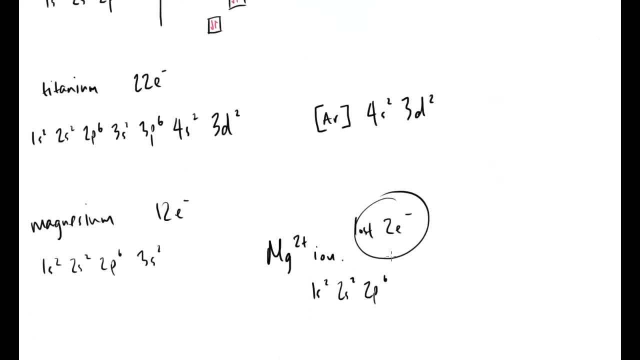 energy, and that makes a bit more sense, i think, when you start to think about what's happening when these electrons are lost in particular. so that's the ions. be aware of that. there are a couple of exceptions to this rule, okay, and i'm not going to go into massive detail about why. 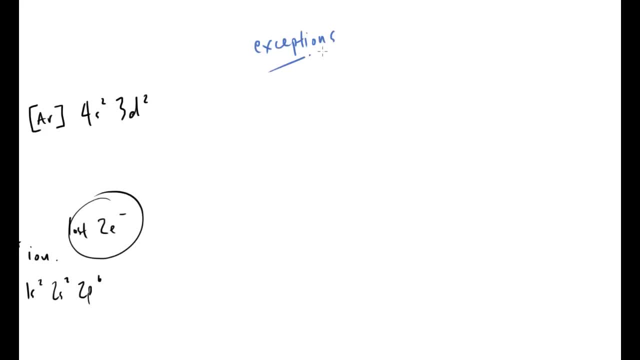 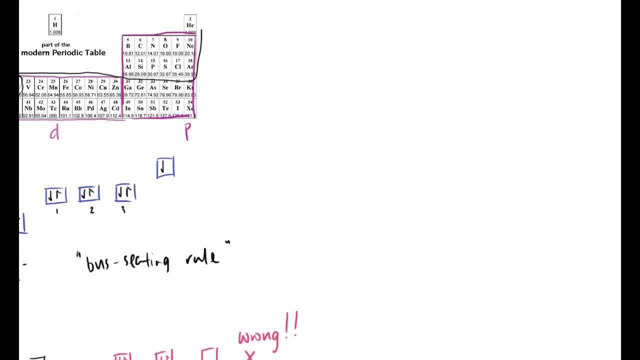 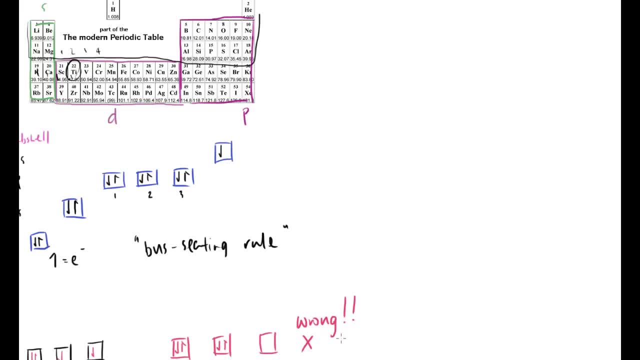 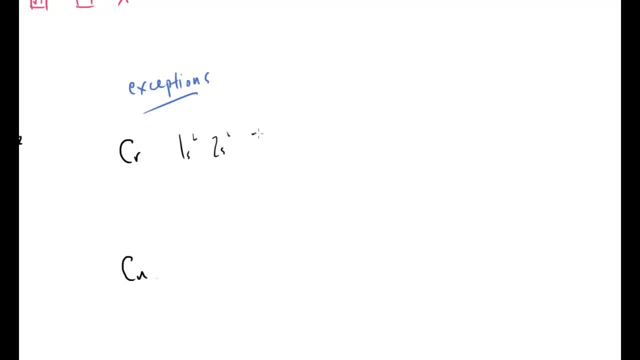 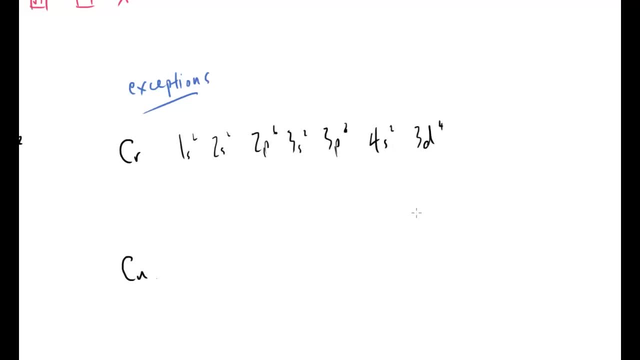 that it's not actually true. okay, that doesn't happen in reality. what we find is that it does this really annoying thing and actually it goes 4s1, 3d5. we're going to start to think about this. the reason it does that is because it takes one of these s electrons and actually puts into a D. 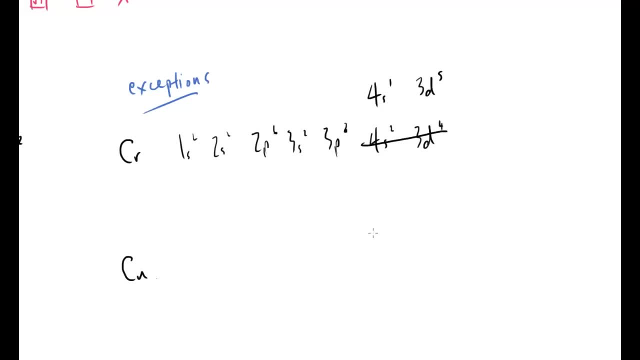 into one of the D orbitals instead, because prior to this we had: there's the forest, there's the 3d. remember that we've got five orbitals for our 3d. we had that and then we had one, two, three, four. what it does is it says: right, I'm gonna get rid of this electron and I'm gonna promote it up into 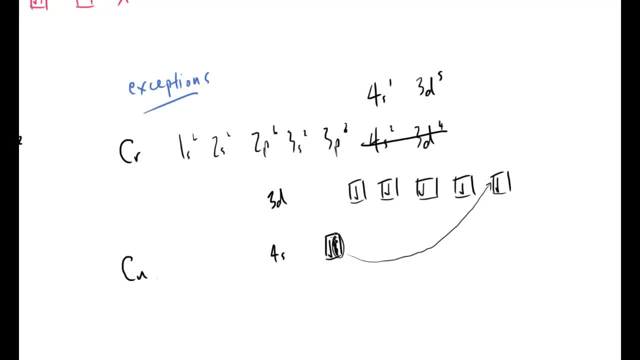 here. so we end up with that there. this one becomes empty, and this is our forest one now and our 3d 5. what this does is it creates a more stable overall structure, having that spread of electrons in those D orbitals. so you're not expected to really understand why it's happening, just that it. 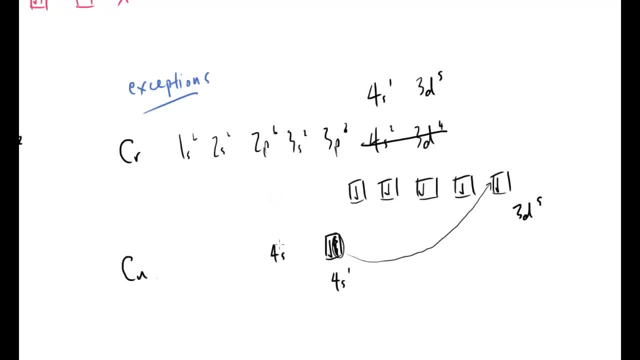 does happen is the key thing there. so I'm just gonna get rid of that very quickly. the other exception there is copper. as you can see, and it's a very similar one. copper should be 4s2- 3d9, but copper being copper being difficult it. 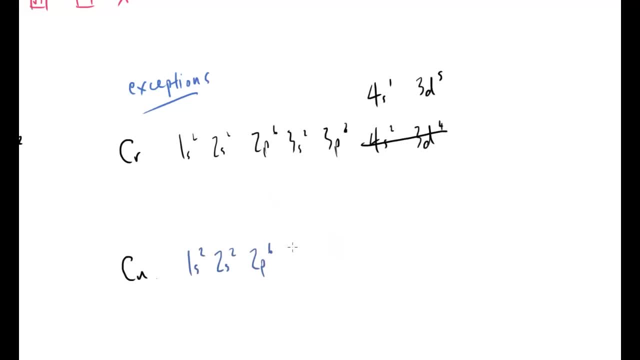 actually goes: 1s2, 2s2, 2p6, 3s2, 3p6. it's a terrible six that there's a six- I apologize- 4s1, 3d10. okay, instead of the 4s2- 3d9 that you would expect again. 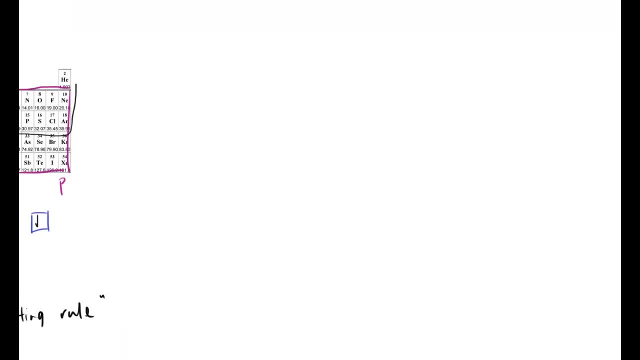 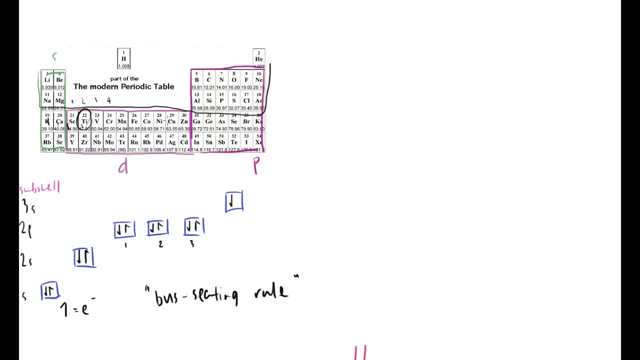 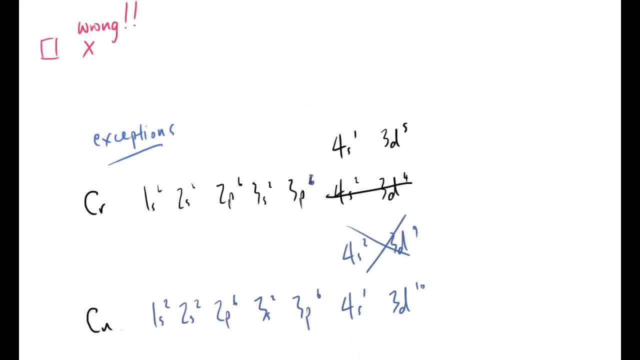 because it then has two in each of the D orbitals, which again makes it gives you more stability. so again, look at this. we would expect one, two, three, four, five, six, seven, eight, nine in the D, but we don't end up with ten and it drops out, gets rid of one of those 4s instead. that's pretty much the. 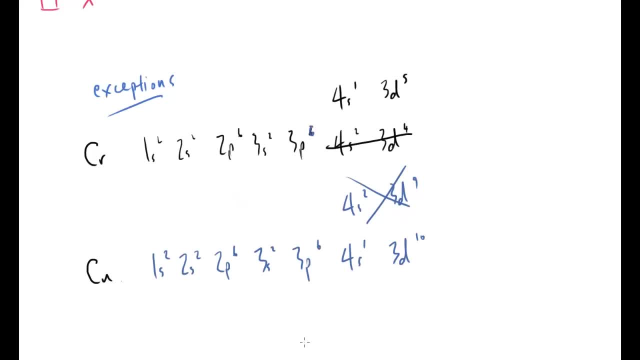 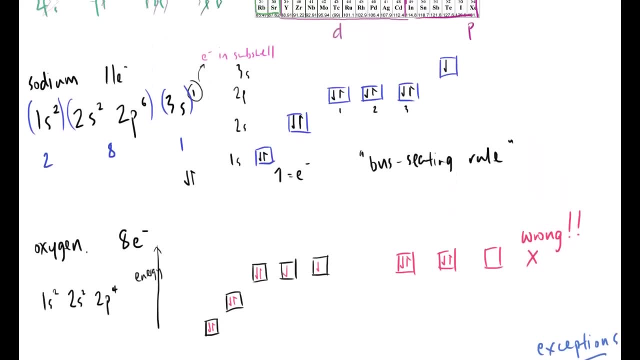 atomic structure, the electron configuration done. it is a strange idea. it's a strange topic. when you start looking into- if you do want to do any research on these various points, like orbitals and rest, you'll realize it becomes incredibly, incredibly difficult. but in terms of the a s, this 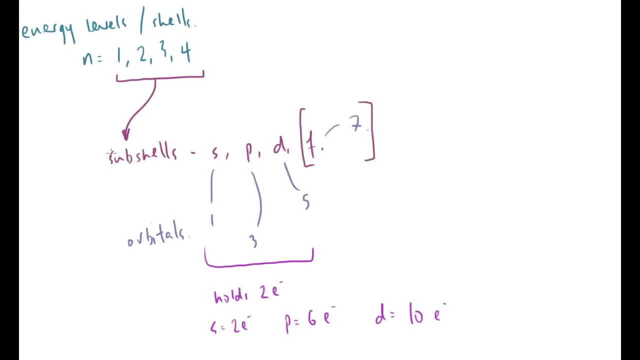 really this little portion here. if I was going to coach you learn anything, it would be this, and then also this little bit of how you, the order you go in, because actually this page here with that all, with that order, will give you everything you need for for electron configurations, particularly the 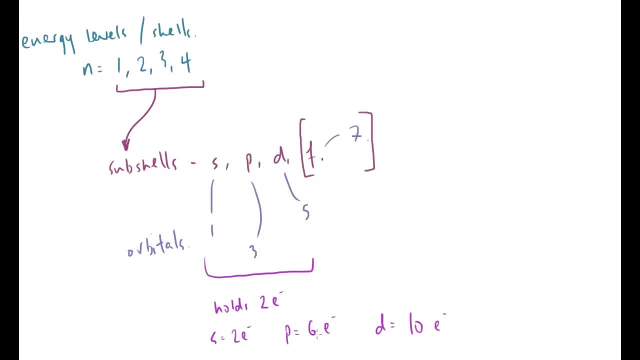 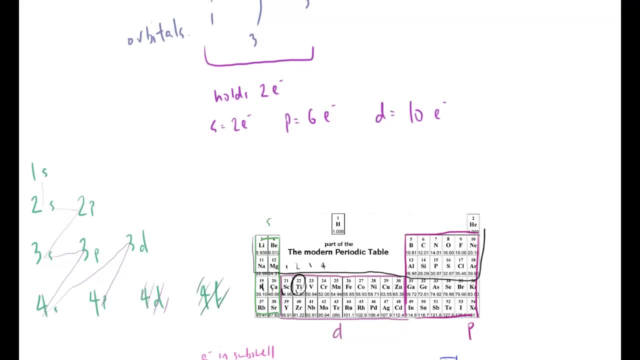 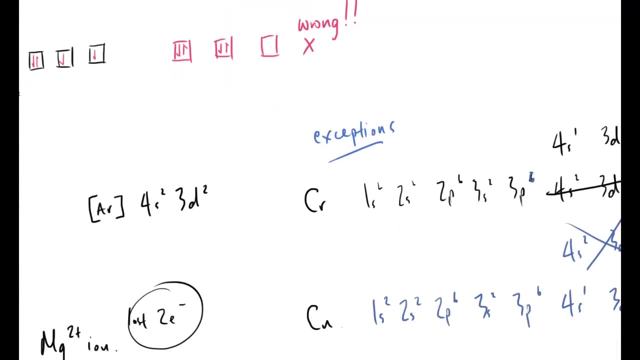 idea of the two electrons being held in the s6 and the P and through ten in the D, and the order then on one, two, three, P, the all the rest, if you can get your head around that, you can name any. we can write down any electron configuration. so I'm going to stop there. hopefully that has been of some of 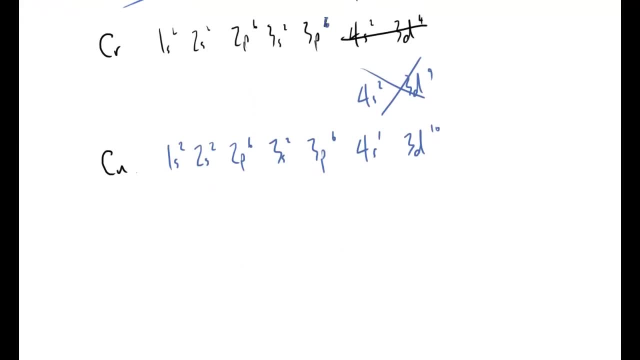 some help. I do. I do hope it has. if I would just do, I'll just goes one quick check for you to say, you know, are you happy that you've done it or how you happy that you understand? write down the electron configuration for sulfur, just to see if you've got your head around it, and then I'm going to. 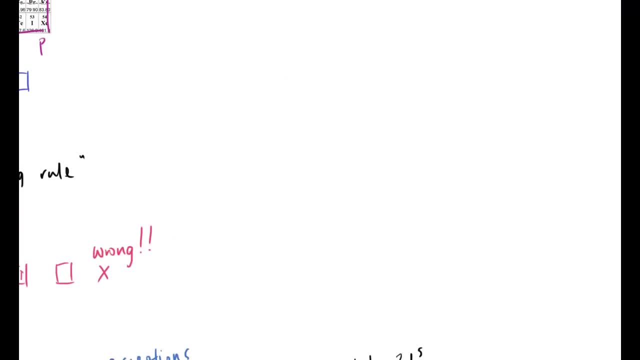 get your head around it and then I'll go back to this one. so okay, so sulfur, hope. at this point you have. you have written that sulfur, 16 electrons. so go down here, off the page six, about the fourth wall, there is that 16 electrons. so we go through 1s, 2, 2s, 2, 2, p, 6. that's taking me to 10, 3s, 2, 2p, so 2, 4, 10. 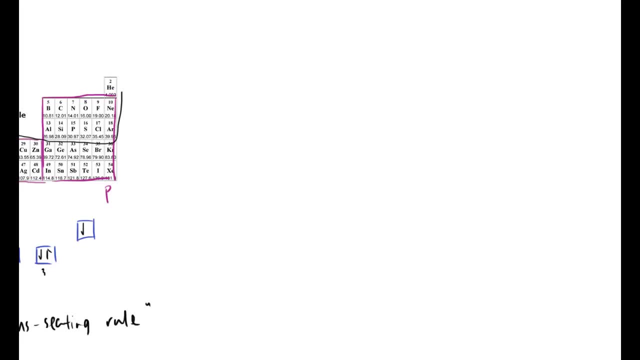 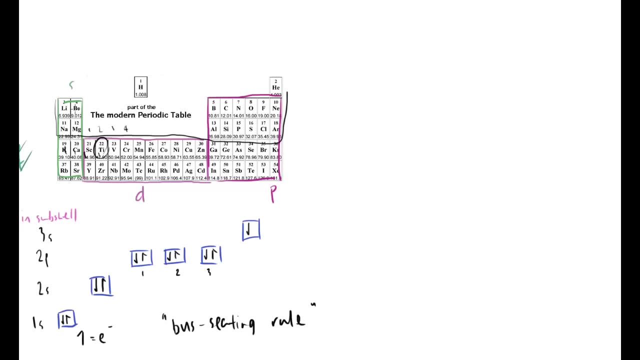 12, 4 And actually an easy way to check this as well. it's really really quite straightforward. Think of these- and you might have seen me doing it earlier on: think of these as separate blocks. So think right, if I'm in here, I must be filling my S2.. 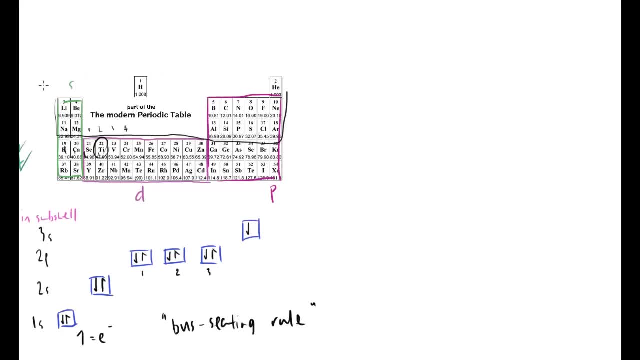 Here it's going to be my S1, and then the 1, 2,, 1, 2, 3, like that Easy check here. sulphur, I'm filling my P, so it's already got the full S. 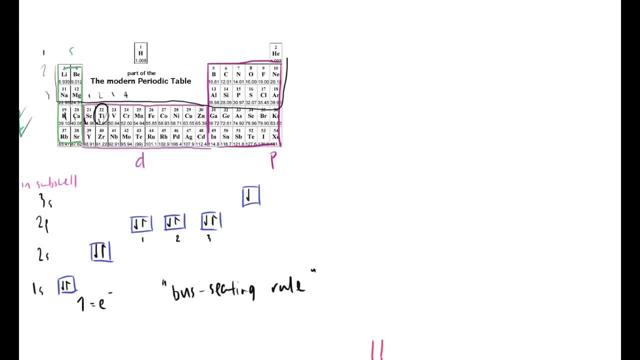 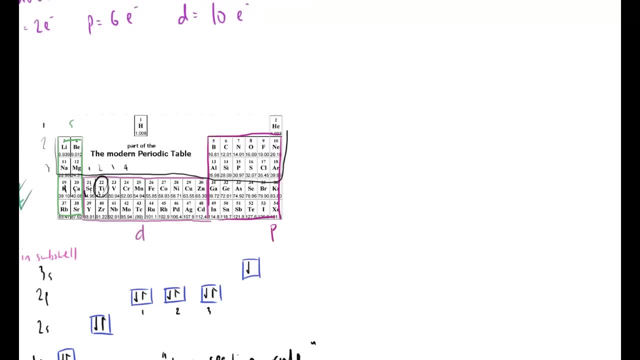 P1, P2, P3, P4. And if I go down here you'll see that's actually true. I have the P4 is what I'm filling. Similar thing's true with the D: D1, D2, D3, D5,- annoyingly- D6, D7, D8,. no, got that wrong, sorry. 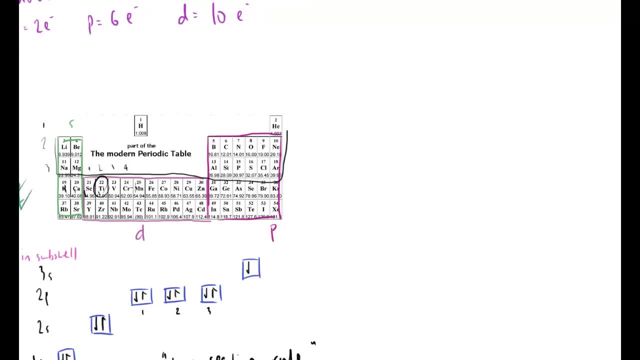 D1, D2, D3, D5, D5, D6, D7, D8, D10, D10.. Okay, so this is a bit more weird from the D, but certainly the S and P Think of them as the S blocks and the P blocks and that's actually a double check there. 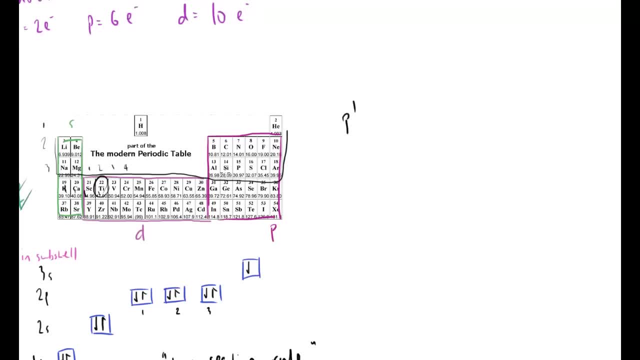 So boring. for example, I know we'll end- We'll end with P1.. Silicon will end with P2.. Nitrogen will end with P3, et cetera, et cetera. So hopefully that's been of some help. 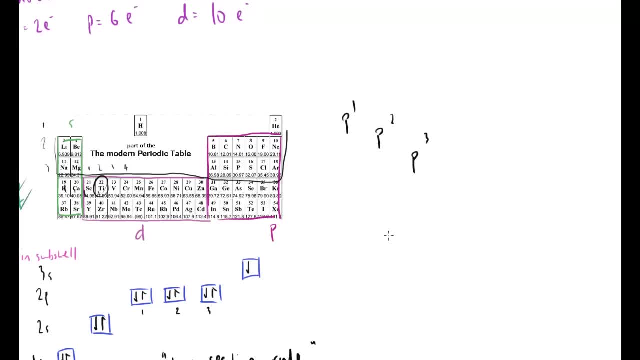 Please let me know in comments if you have any queries or any questions. And yeah, there you go. Electron configurations. 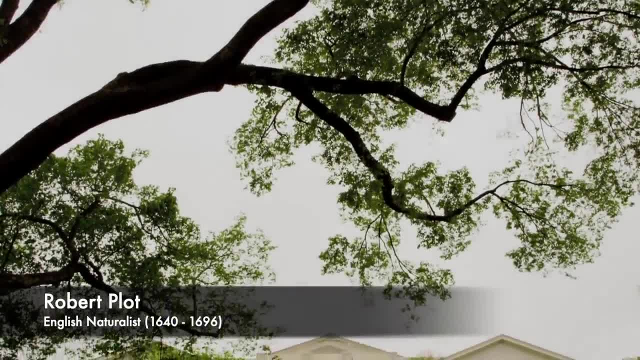 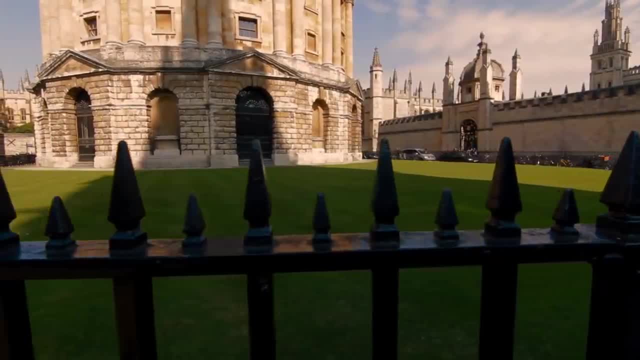 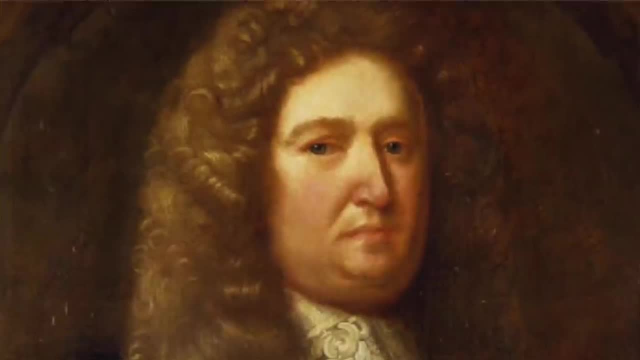 Reverend Robert Plott is an educated man, a professor of chemistry at the prestigious University of Oxford, but he is as excited as a child at Christmas. when new parcels arrive In 1677, he hurries around the grass quad of University College and bursts through the